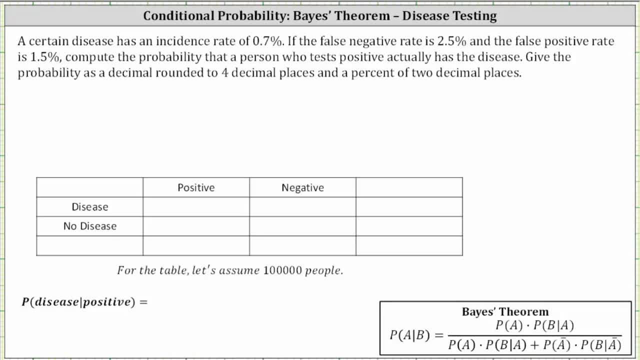 Welcome to an example of conditional probability. We will first determine the probability using a table and then also find the probability using the formula for Bayes' theorem. A certain disease has an incidence rate of 0.7% If the false negative rate is 2.5%. 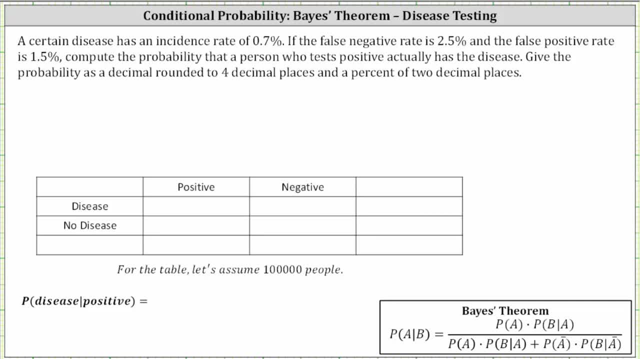 and the false positive rate is 1.5%, compute the probability that a person who tests positive actually has a disease, which means we are looking for the conditional probability, the probability a person has a disease given they test positive. To complete the table, we will assume 100,000 people. 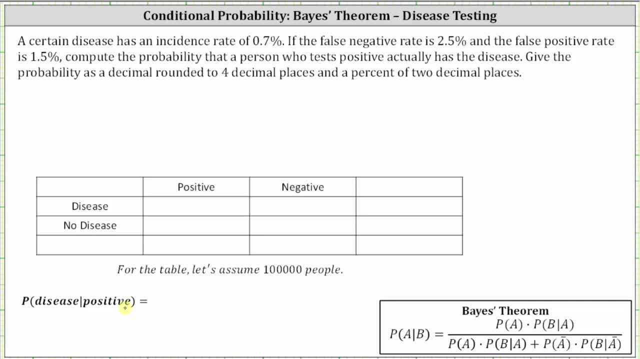 So, to begin, because a disease has an incidence rate of 0.7%, we need to find 0.7% of 100,000.. To do this, we convert 0.7% to a decimal and multiply by 100,000,. 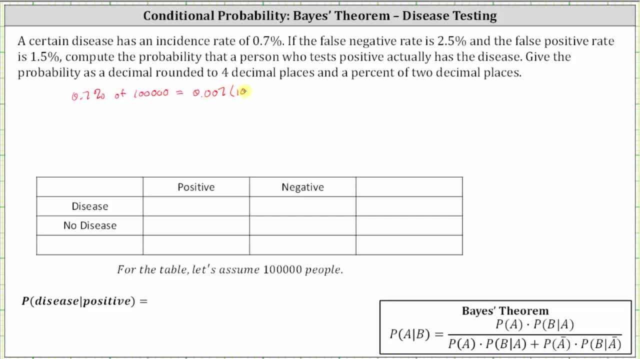 which gives us 0.007 times 100,000.. 100,000, which is equal to 700.. So the total for the row that represents those that have the disease is 700,, which would be this cell here, which means the number of people. 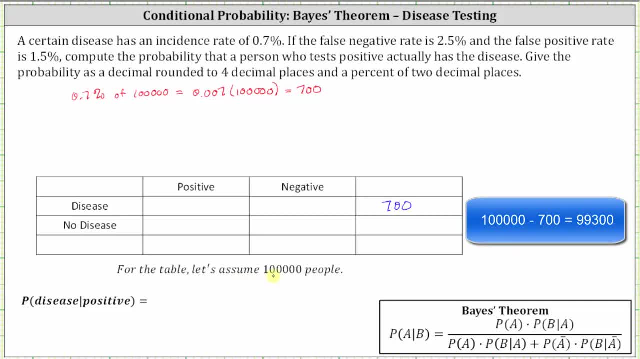 that don't have the disease or no disease, would have to be 100,000 minus 700, which is 99,300.. This is the total for the number of people that have no disease. Next, the false negative rate is 2.5%. 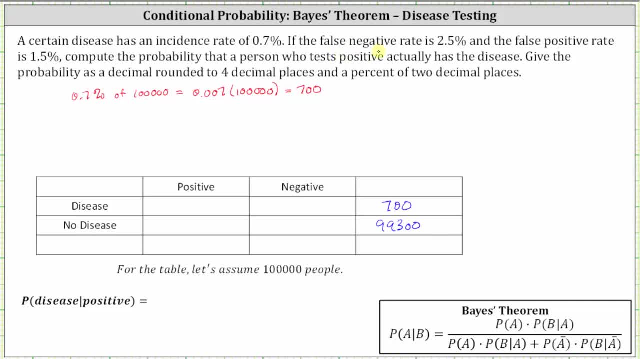 False negative means the person tests negative but actually has a disease And therefore the next step is to find 2.5% of the 700 people that have the disease. So 2.5% of 700 is equal to 0.025 times 700,. 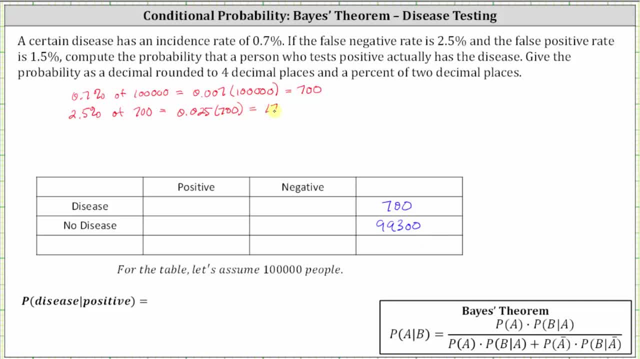 which is equal to 17.5.. So 17.5 represents the number of people that have the disease. 17.5 represents the number of people that test negative but actually have disease, which goes in this cell here, And therefore the number of people. 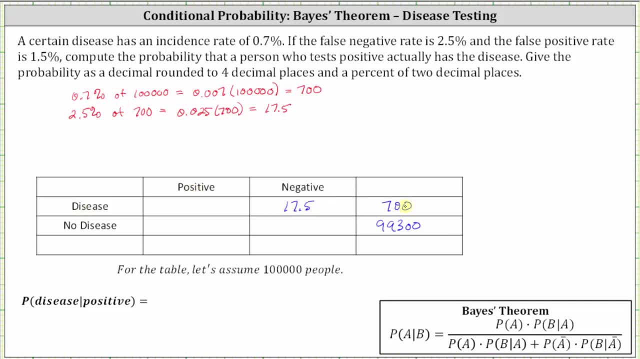 that have the disease, that test positive would have to be 700 minus 17.5, which is 682.5.. Now I know we can't have a decimal part of a person, but to model the situation we are going to use decimals in the table. 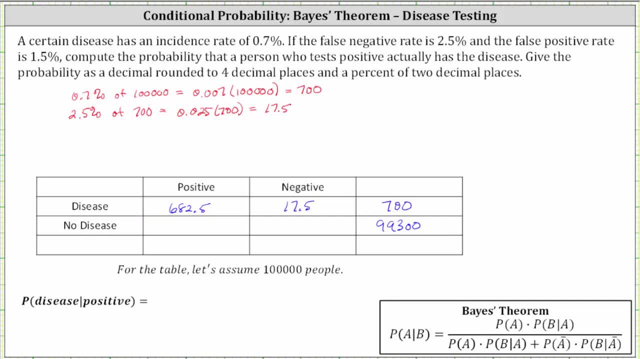 And again we obtained 682.5 by taking the total number of diseased people of 700 and subtracting those that tested negative or 17.5.. Next, we're told the false positive rate is 1.5%. False positive means they tested positive for the disease. 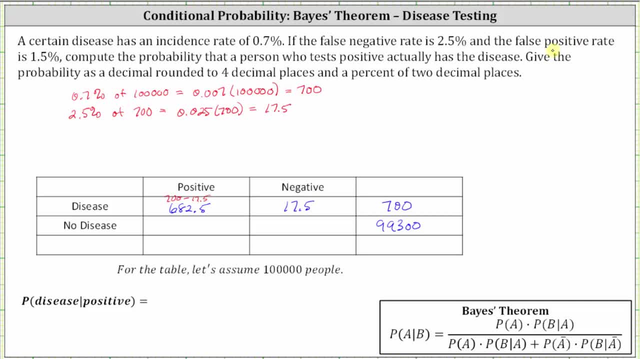 but did not have the disease. which means the next step is to find 1.5% of the people with no disease, or 1.5% of 99,300, which is equal to 0.015 times 99,300 but is equal to 1489.5. so again, 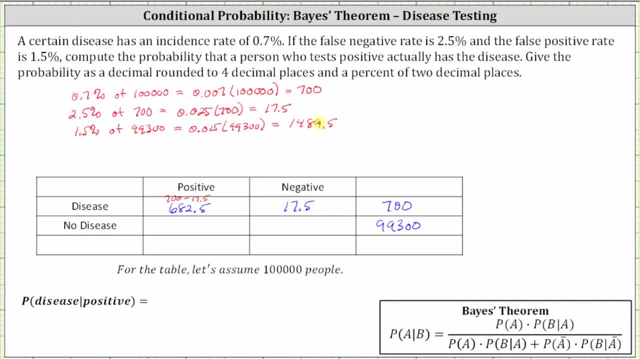 this would be the number of people that test positive, that don't have the disease, which would be the amount in this cell here, and therefore the number of people that don't have a disease that test negative would have to be 99,300 minus 1489.5, which is equal to 97,810.5. 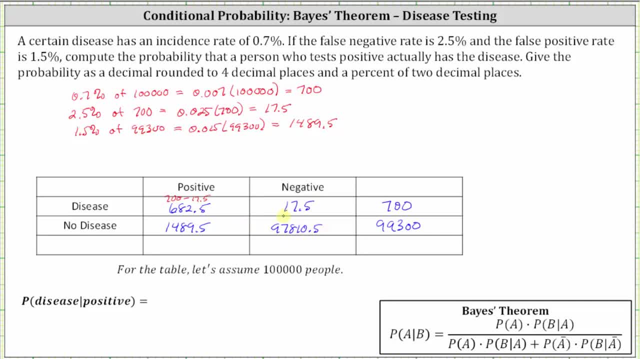 again. this value came from taking again. this value came from the total of people with no disease of 99,300, and subtracting those that have no disease that test positive, which is 1489.5. the next step is the sum of the columns: the positive column, the negative. 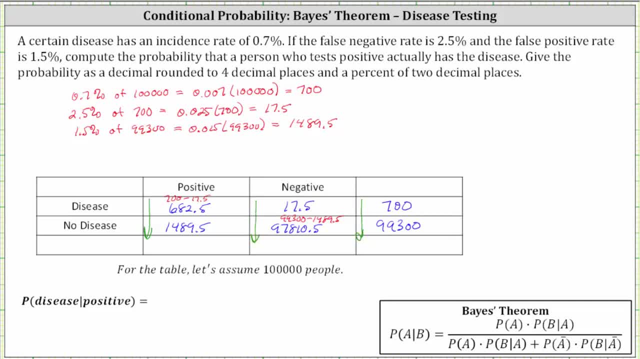 column and the total column. well, we know the sum of the total column is going to be 100,000, the sum of the positive column is 2172 and the total of the negative column is 97,828. if we total, this last row will also get a sum of 100,000, and now we have the. 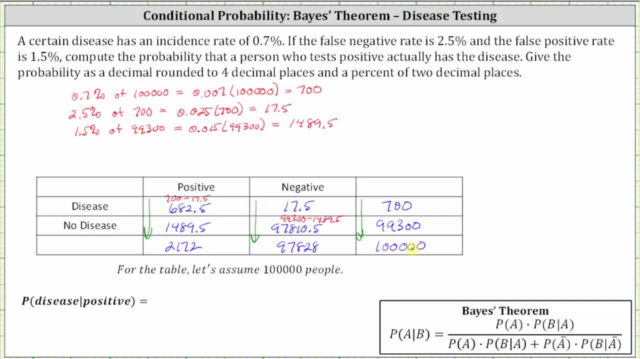 information from the table we need in order to find the probability a person has a disease, given they test positive. because is given they test positive, we are only concerned about the positive column. of the 2172 people that tested positive, 682.5 actually have the disease, which means the probability a person has 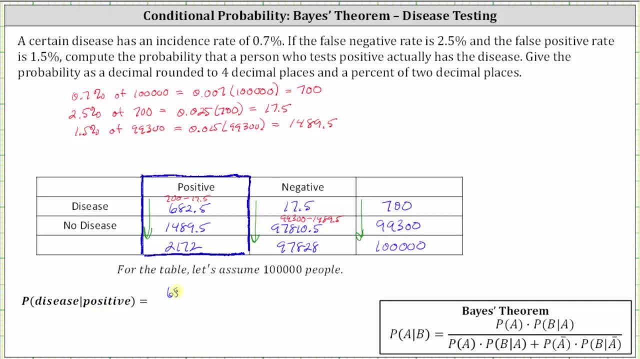 has a disease. given the test, positive is equal to 682.5 divided by 2172,, which is a decimal, rounded to four decimal places, is 0.3142,, which is a percent to two decimal places, is 31.42%. And now let's find the same probability using the: 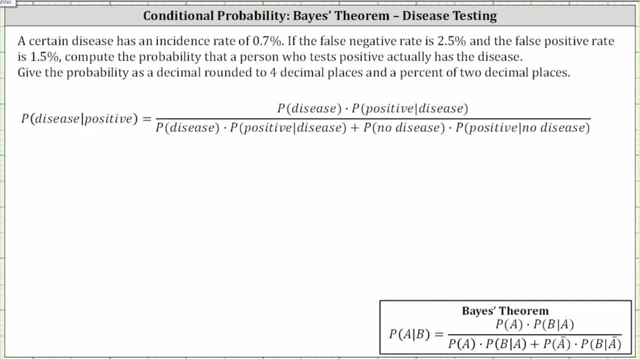 formula for Bayes' theorem on the next slide. So the first thing to recognize when applying the formula is event A, in our case is the event of having the disease, and event B is the event of testing positive. So applying the formula, 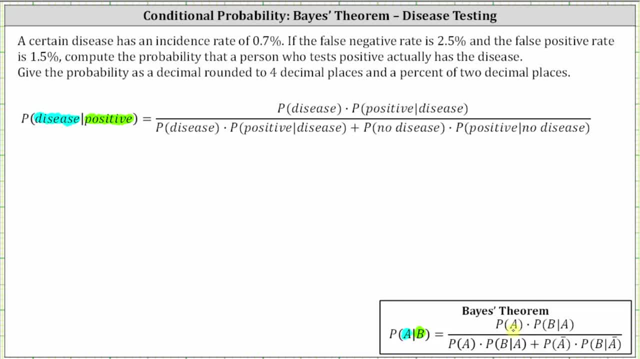 for Bayes' theorem. the probability of A is a probability of having the disease. the probability of B, given A is the probability of testing positive, given given they have the disease. in the denominator again we have the probability of disease times the. 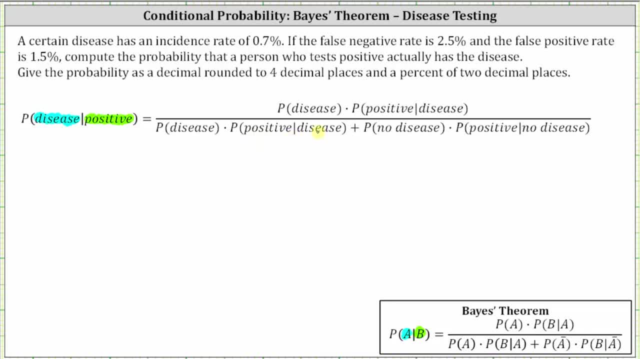 probability of testing positive, given they have the disease. Notice how we do have some repetition in the numerator and denominator here, in this product as well as this product. And then we have plus the probability of not A, which is a probability of no disease, times the probability of B given not A, which is a. 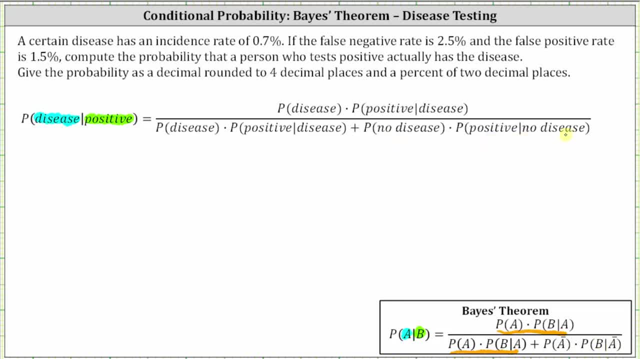 probability of testing positive given no disease. And now let's find these probabilities In the numerator. we have the probability of disease, which is the incidence rate of 0.7 percent or, as a decimal, 0.007.. And then we have times the probability of testing positive given. 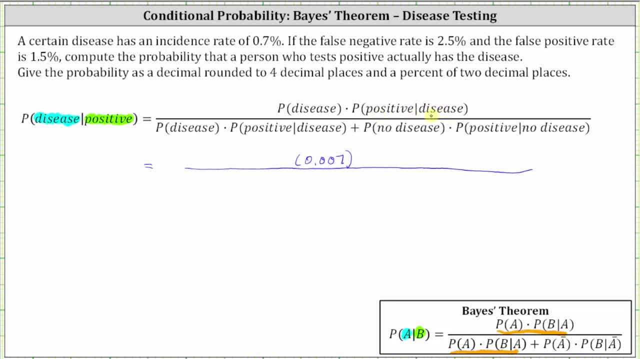 they have the disease. This is going to be equal to 100 percent minus the false negative rate. Remember, the false negative rate is the percent that test negative that actually have the disease, which means 100 percent minus 2.5 percent. 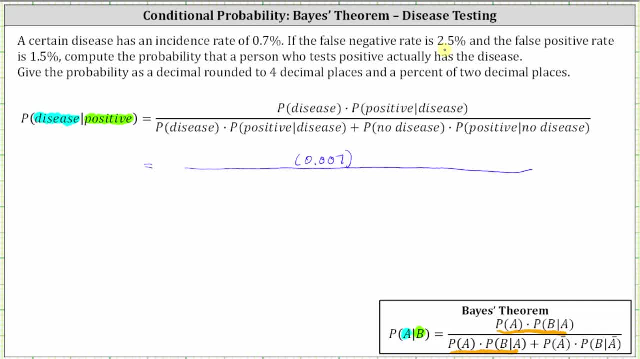 or 97.5 percent gives us the probability a person tests positive, given they have the disease. 97.5 percent as a decimal is at 0.975.. In the denominator, again we have the probability of disease, which is again 0.007 times again the